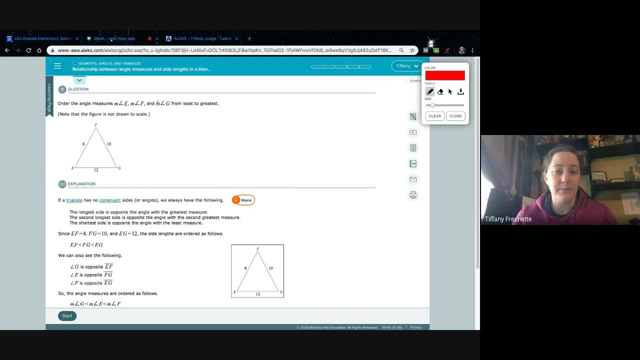 of angle G, Only see M- and then the angle symbol- That's how you say it: Measure of angle from least to greatest. Note that the figure is not drawn to scale, So they don't actually want you to measure the angles or anything like that. They want you to pay attention to the relationship So and down. 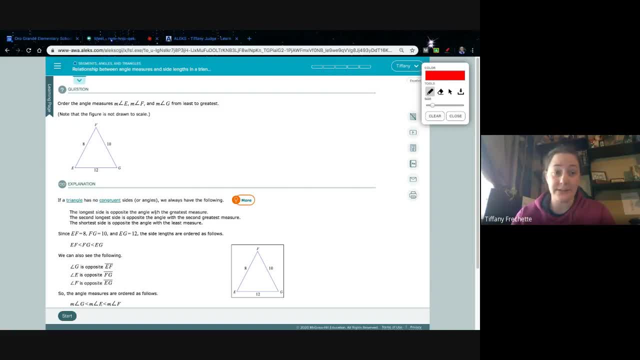 here they give you notes. If you are not reading the notes or the explanation pages, you need to start reading the explanation pages And you should start taking some notes on them. It is definitely important to pay attention to what's going on. So if a triangle has no congruent sides, 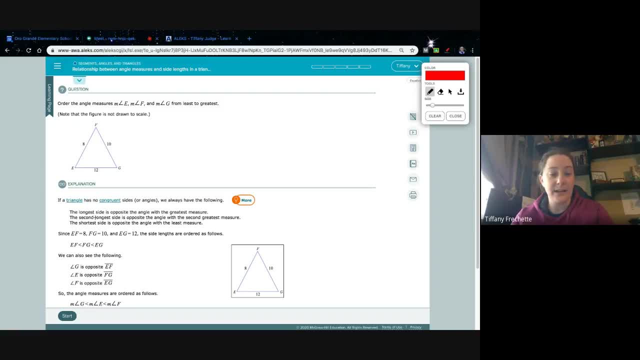 or angles. we will always have the following: So it gives us these three kind of rules here like this. I'm going to click clear because I started writing on that one: The longest side is opposite the angle with the greatest measure. The second side is opposite the angle with the second greatest. 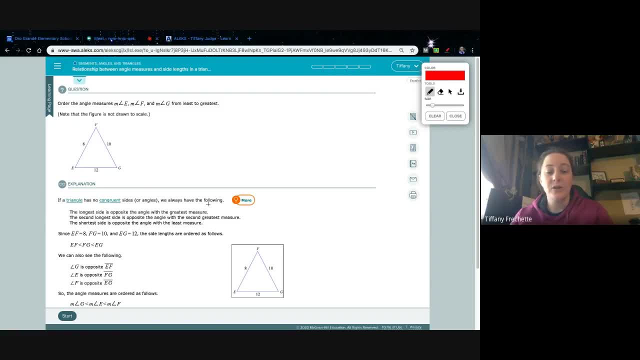 measure And the shortest side is opposite the angle with the least measure. So it's just a relationship we see. So if we want to go from least to greatest, I can simply say: well, what's my smallest side? My smallest side is 8.. So I'm going to go 8. And I'm going to go straight across from 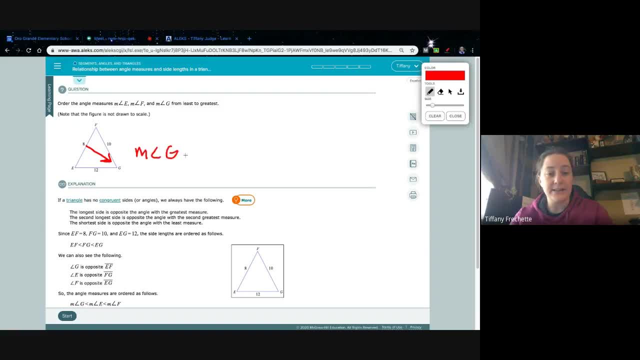 that. So the measure of angle G is the smallest. And then I go to my next side. So I went smallest. Now I want to go one bigger or the next Biggest- I guess I'm saying that funny- So 10.. So 10 is across from E, So that means that the 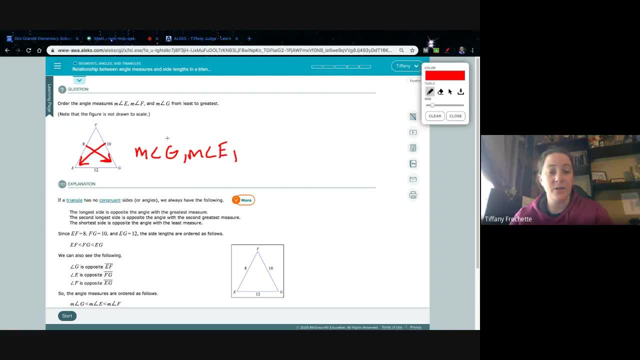 measure of angle E comes next to my list, So G is the smallest. E is kind of my middle measure here And then the largest angle will be across from my largest side. So 12 is my largest side. I go straight across And there's my angle. So the measure of angle F is my largest side And this 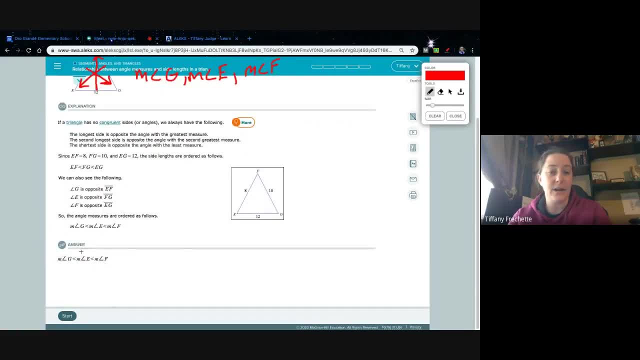 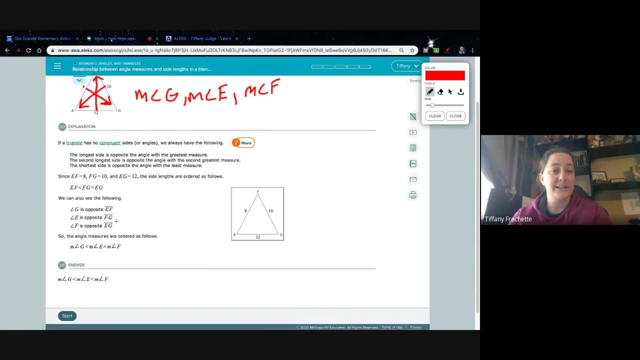 is simply what they want you to do. So if I scroll down here, you can see this is what they're having to do. And if you notice, the page marker only works a little bit So it stays with the page, And then all of a sudden it doesn't know what to do with the blue And it just goes with the blue. 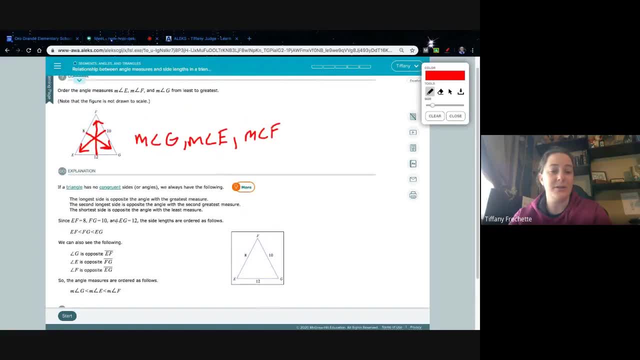 because it's on that part of the page So it doesn't understand to keep going up. But it's a cool tool but it's limited, So I'm going to clear it. I'm going to go to the next page. Oh, I have. 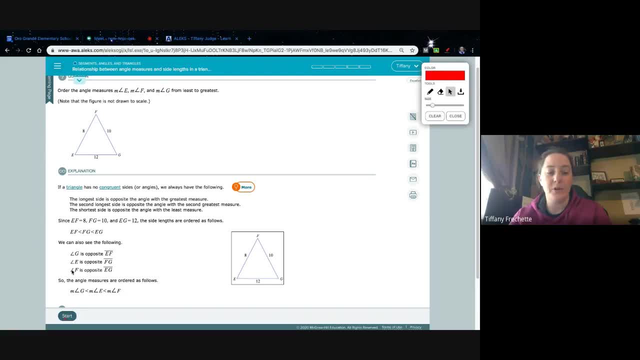 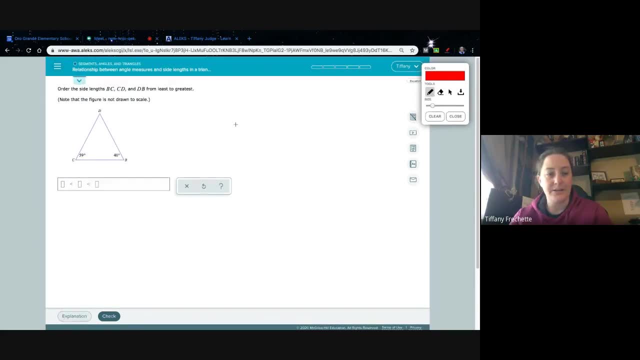 to make sure I click my pen tool or my cursor tool, or it won't work. It'll keep marking So you can see I put a dot down there, All right? So the other thing which we were talking about, the side lengths on the last page, it's the 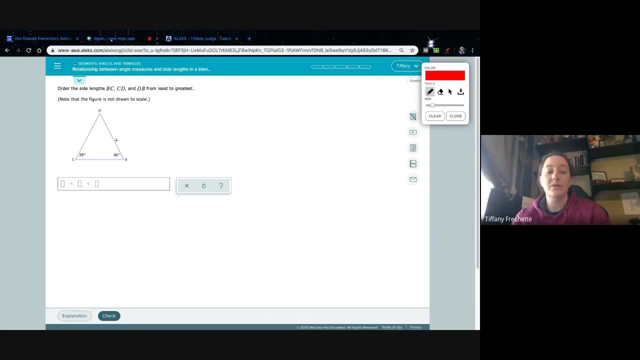 same thing is true with the angle measures. So this time they're giving us angles. So the largest angle is across from the largest side. The smallest angle is across from the smallest angle. So sorry, the smallest side is across from the smallest angle. I'm not sure if I said that correctly. the 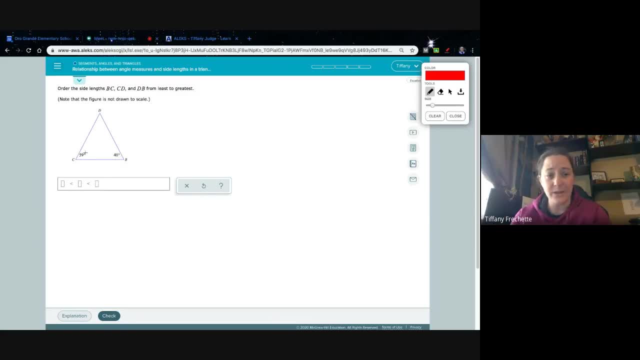 first time. So one thing we do need to know is we need to know all three angles. So we need to know all three angles if that's what we're using, And I hope you remember that the angles of a triangle always add up to 180 degrees, Always, always, always. So then we figure out: what do we have? What? 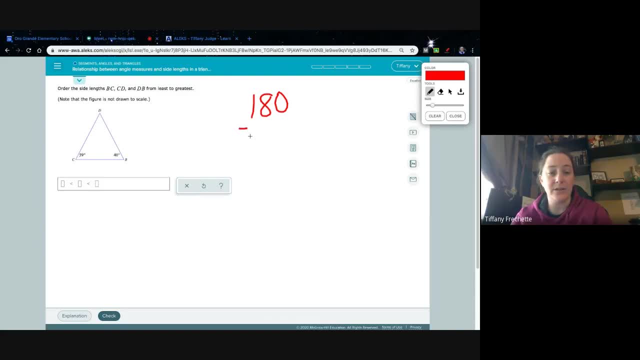 are we using of the 180 degrees. So I'm going to add those two together and I get 99, because 59 plus 40 is 99.. I'm going to subtract. So here's I'm borrowing: Do, do, do, do, do, do, And I get and I have. 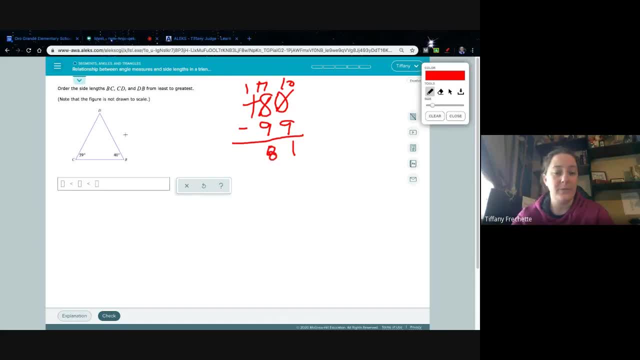 to borrow again, I get 17 and I get 8, so I have 81. so this is 81 degrees and that is quite a bit larger than what that angle looks like. so again, make sure you understand it's not drawn to scale, they do not. 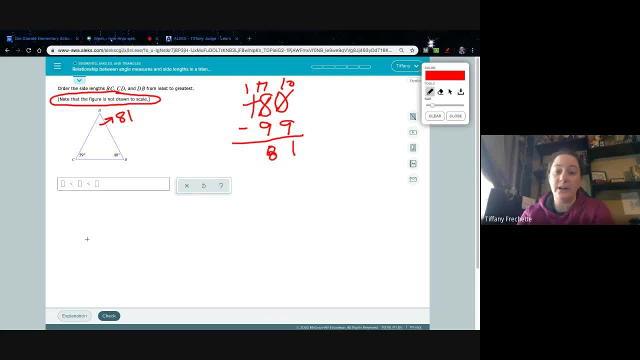 want you in any way to try to measure these with a protractor or anything like that. they want you to literally do the math on figuring this out. how does it work? so we know, if we add these two together, we get 99, and then if I subtract from 180, I get 81. so now we have our three angles here, and 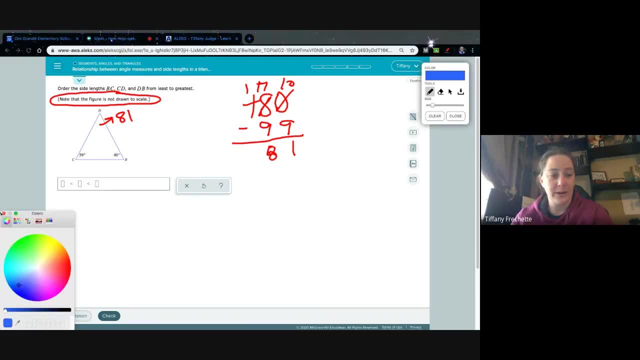 I'm gonna switch my color up, switch it up to blue here. why not close that? whoops did not mean to maximize it, I wanted to close it, okay. so we want it from least to greatest. so I want my smallest angle first. so I'm going to do my smallest angle first. so I'm going to do my smallest angle first. 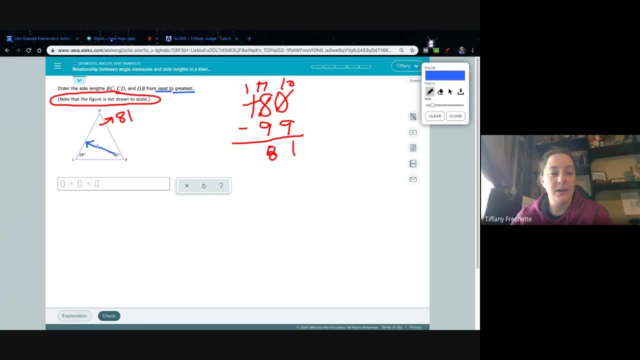 gonna go my smallest and I'm gonna go across. and when I write my side length I need to make sure I have both letters. so my smallest side- whoops, I have to hit my cursor, silly me- is CD or I could have put DC, it would have been fine. but just make sure a line needs two letters or two points in. 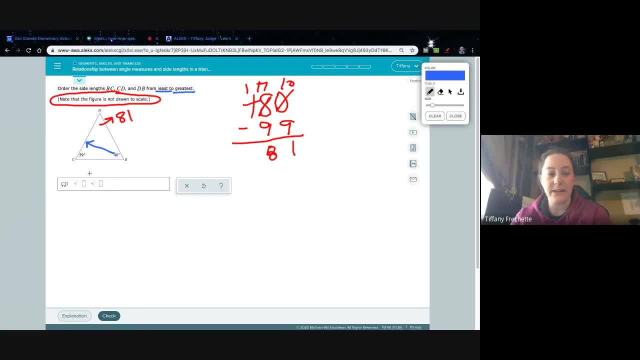 order to be a line. alright, my next one is 59 here, so I'm gonna go across to this one. so this is B, D or DB. either way, I hit my cursor- again DB, and then I have my last one, which is 81, which is very large. 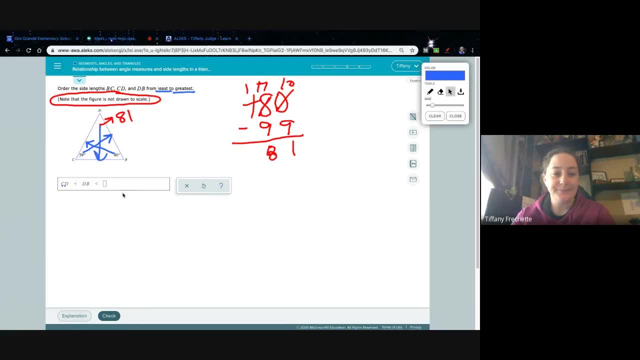 here. I'm gonna go straight down. so I have either CB or BC- I can say it either way- and I click check and I got a point: yeah, we're good, all right, I'm gonna click clear, take all that away next. so we're starting in blue here. now they're giving me the size lengths, so I want to go back to. I want to. 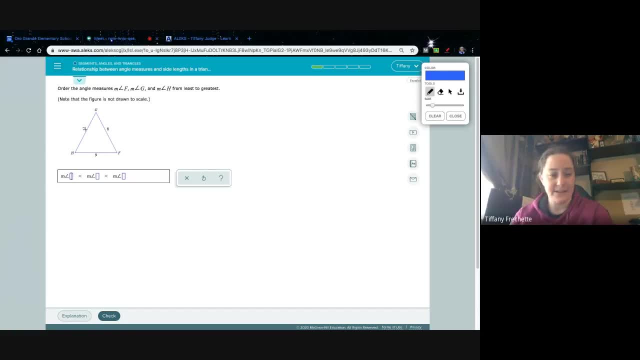 find my smallest side, which is sit. excuse me, it's seven. I'm gonna go straight across. so F is my smallest side and I'm gonna go ahead and type in F. so they're not making you put measure of angle, they just want you to type in the F and the next one. so seven was the smallest, the next one would: 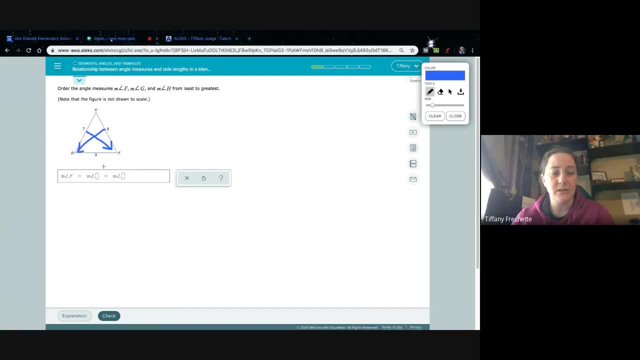 be eight, so I'm gonna go across here to H and I'm gonna type in H. all right, and my last one. there nine is definitely the biggest side, so it's across from my biggest angle, so I'm gonna type in G. click check, yeah, we got another one, all right. 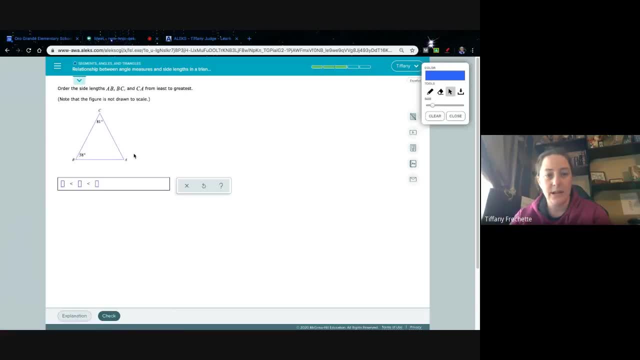 clear. and next: okay, so we need to do our angle measures again because they're giving us angles. so again we start. we know we have a hundred eighty degrees. we know we have a hundred eighty degrees. okay, so we need to do our angle measures again because they're giving us angles. so again we start. we know we have 180 degrees.